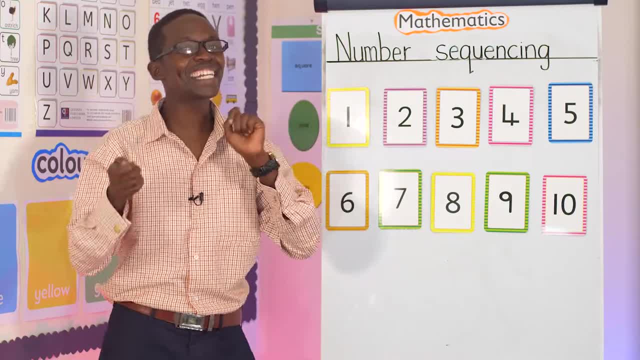 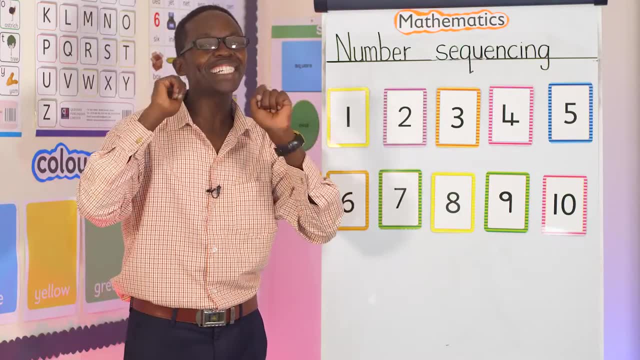 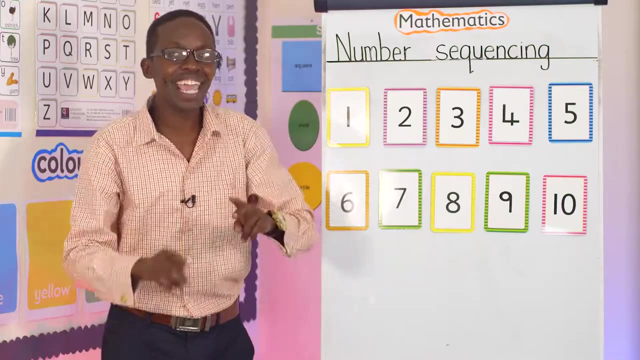 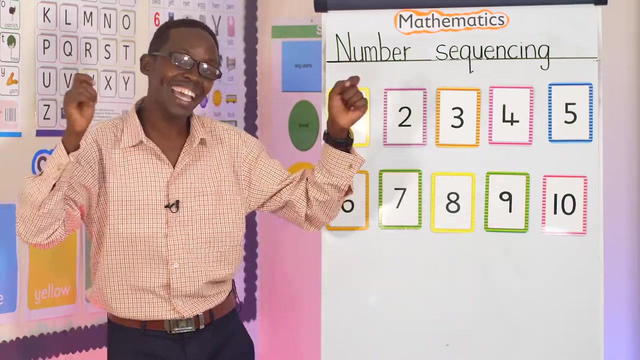 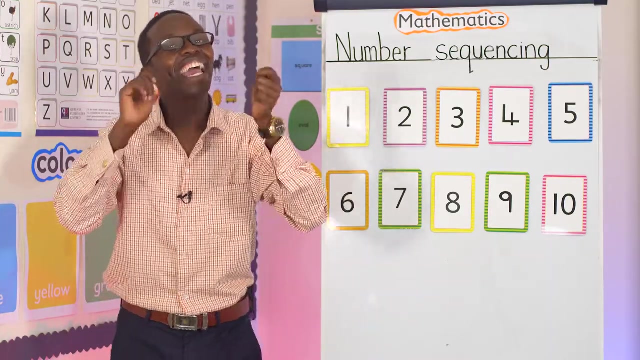 Shake, shake the mango tree, the mango tree, the mango tree. Down fall the mangoes One, two, three and four, Five, six, seven, eight, nine, ten. Shake again Down, fall the mangoes Again. Shake, shake the mango tree, the mango tree, the mango tree. 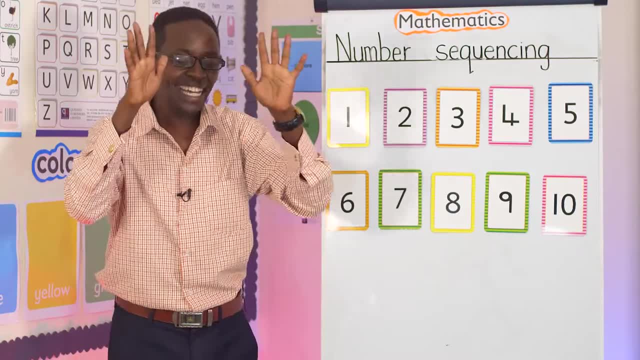 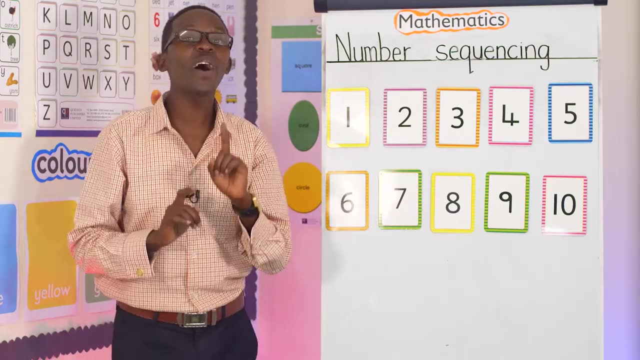 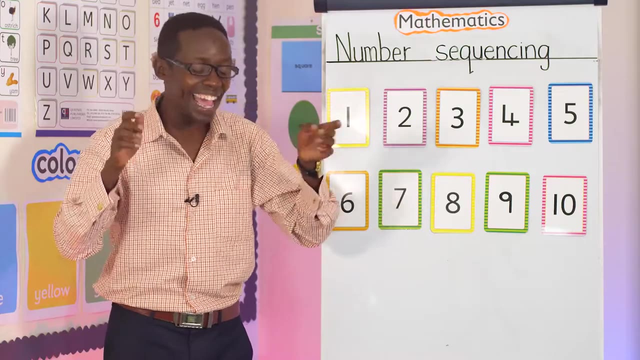 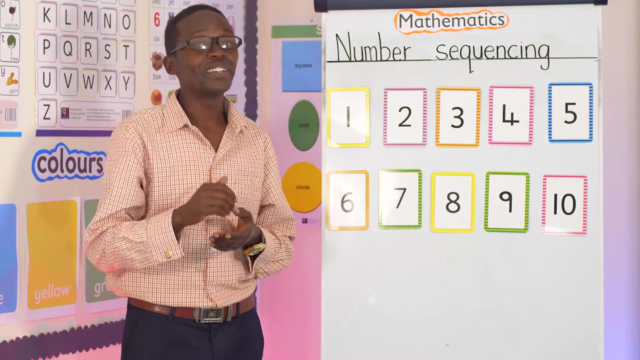 Shake, shake the mango tree Down, fall the mangoes. down for the mangoes: one, two, three and four, five, six, seven, eight, nine, ten. shake again down for the mangoes. do you like mangoes? good, now i want us to clap one up to ten. 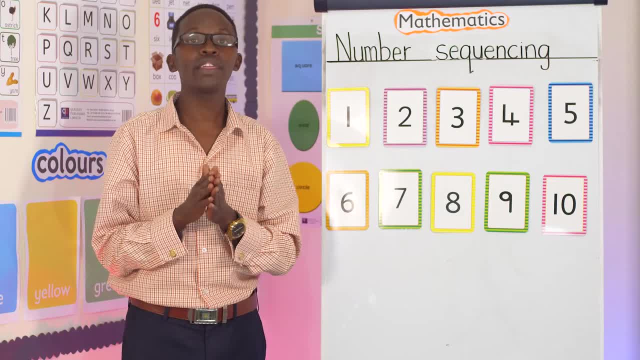 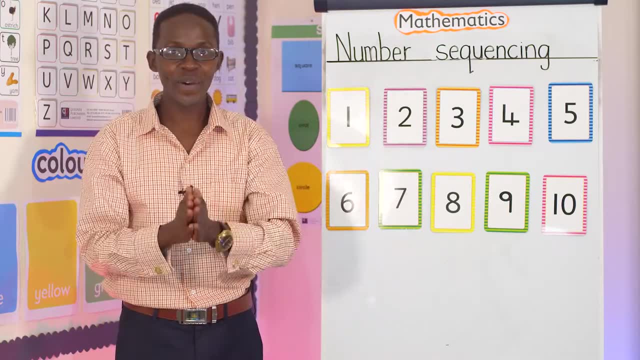 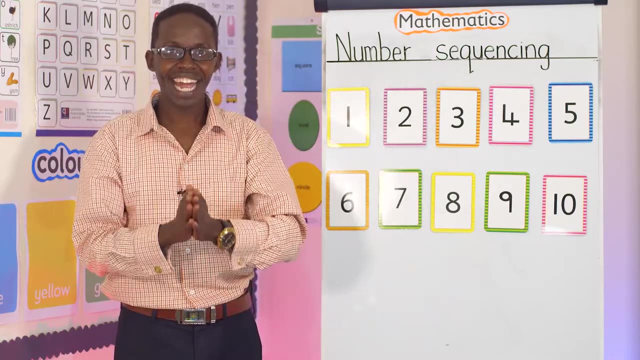 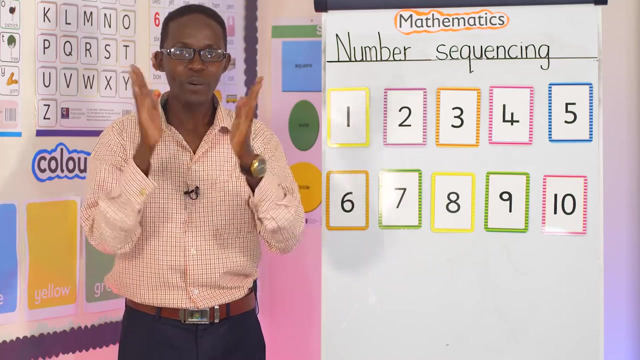 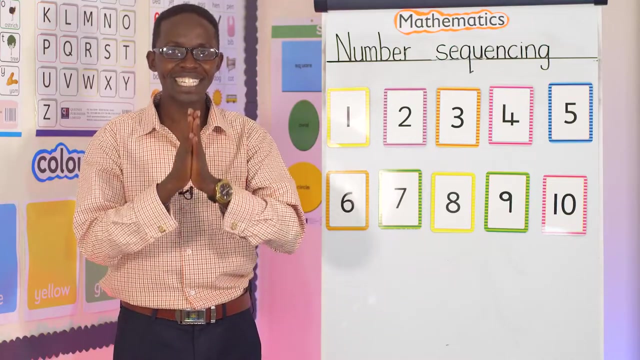 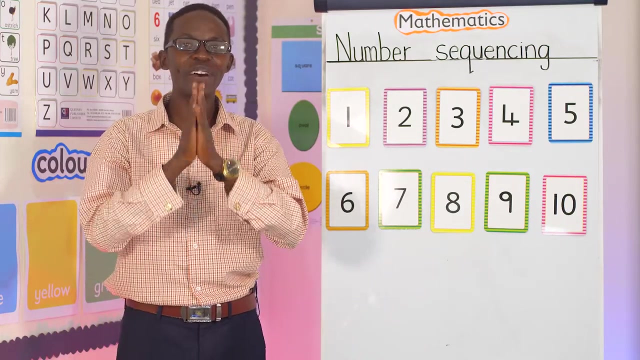 so you know numbers, let's do together: one, two. one. two, three, four, five, six, seven, eight, nine, ten. can we clap again? let's go, let's start again. one, one, two, three, four, five, six, seven, eight, nine, ten. good boys and girls, that's wonderful. i want us. do you know how to jump? 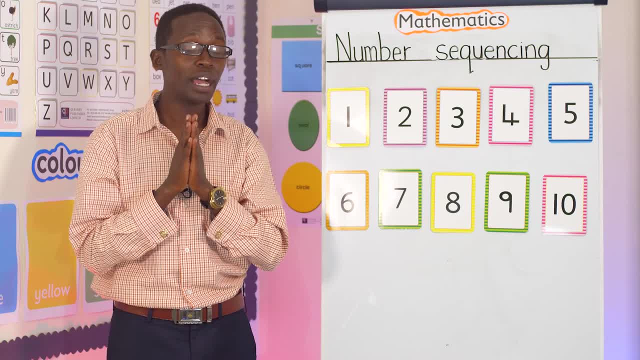 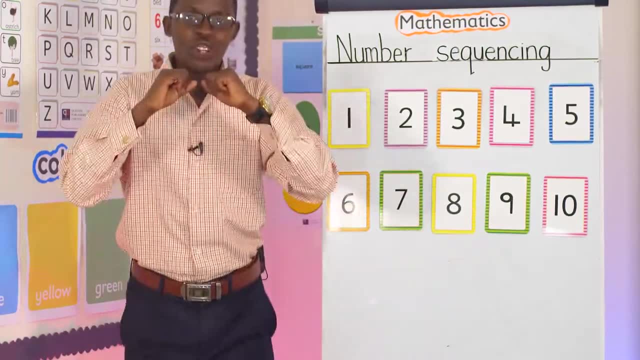 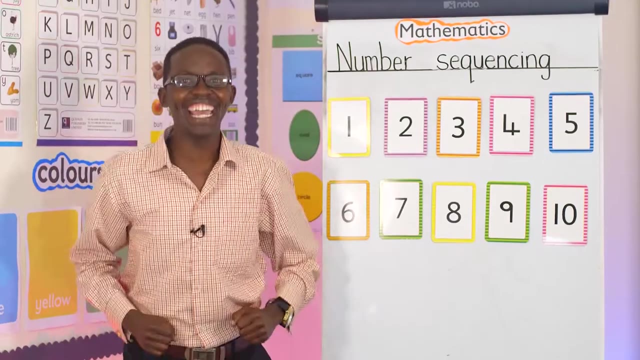 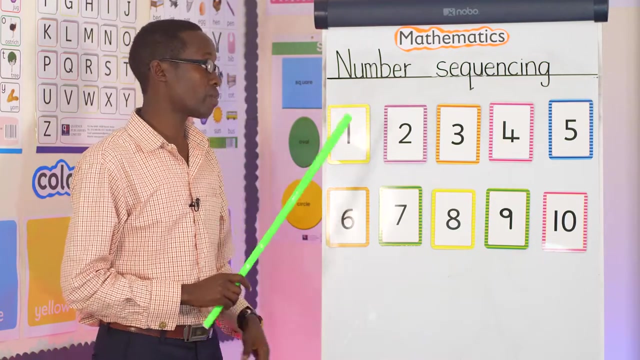 number one to ten. can you be able to jump? i look at me jumping. number one to tap to ten. one, two, three, four, five, six, seven, eight, nine, ten. aha, that's wonderful. now look here, i have numbers on my board, okay, and i want us to. 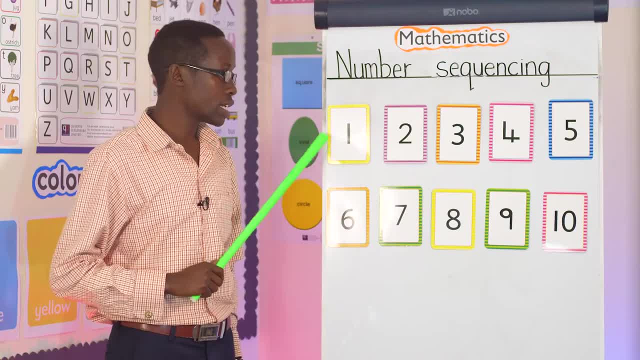 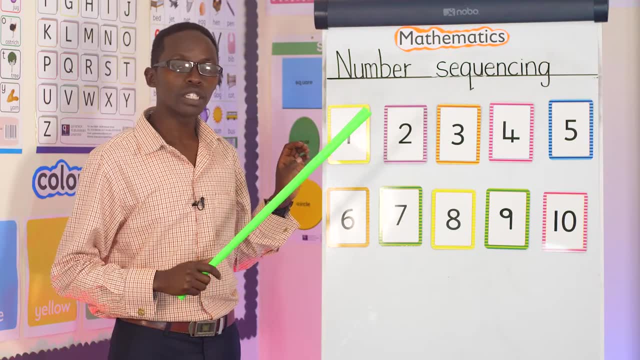 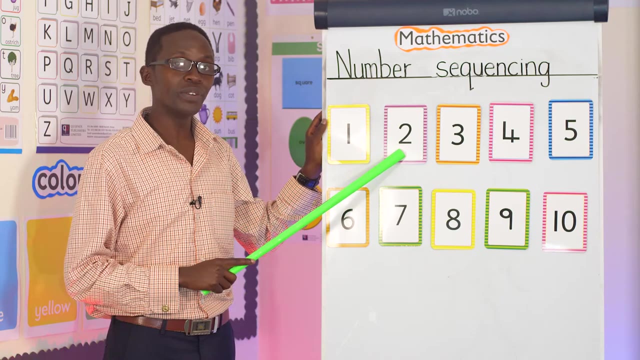 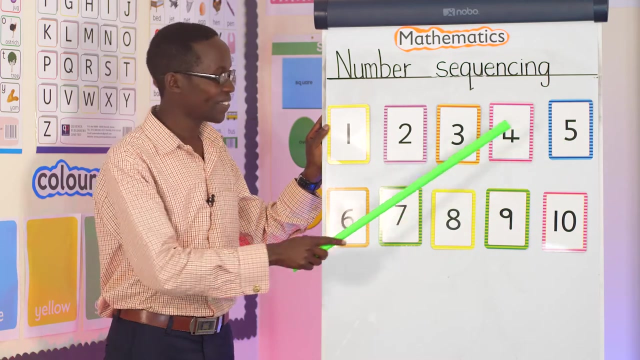 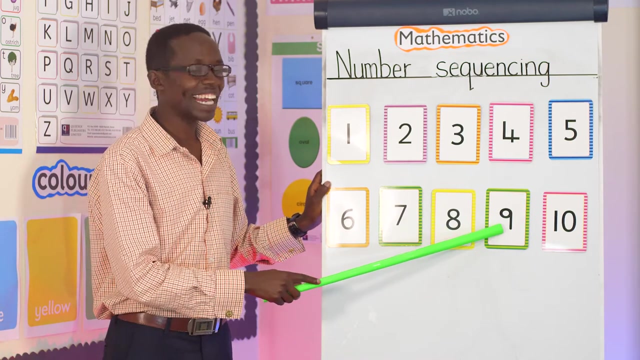 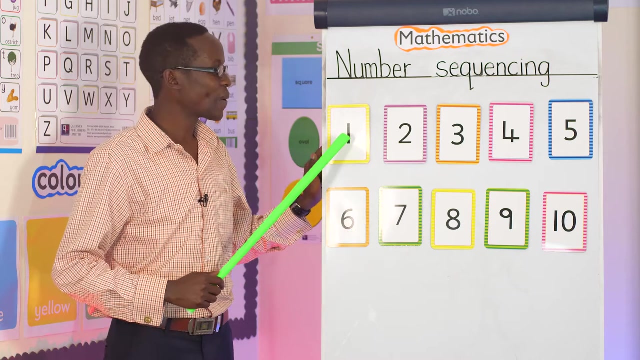 come at all to read, and you read loudly, isn't it? can you start number one? can you see them? can you see here? look here, hey, teacher david, is he look here? good, can you see one, two, three, four, five, six, seven, eight, nine, ten. that's wonderful, can we? can you read again: one, two, three. 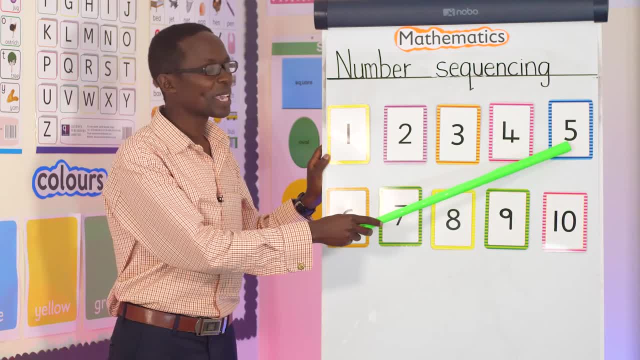 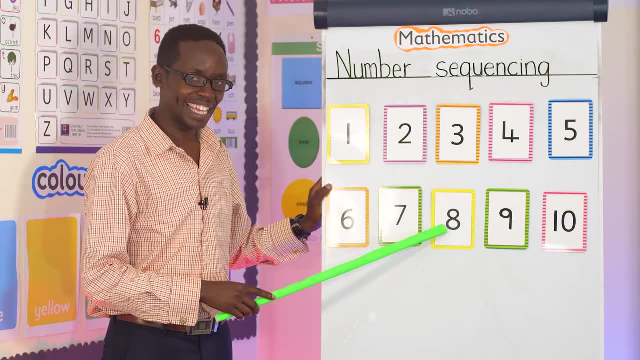 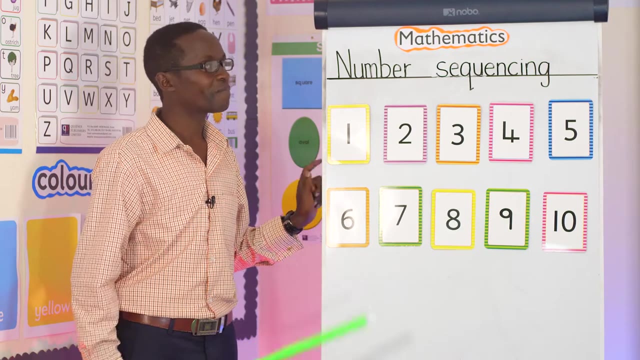 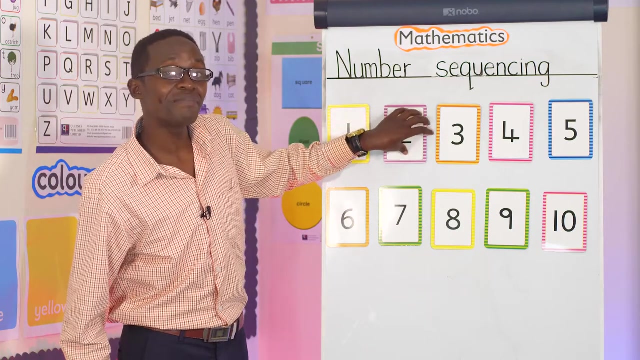 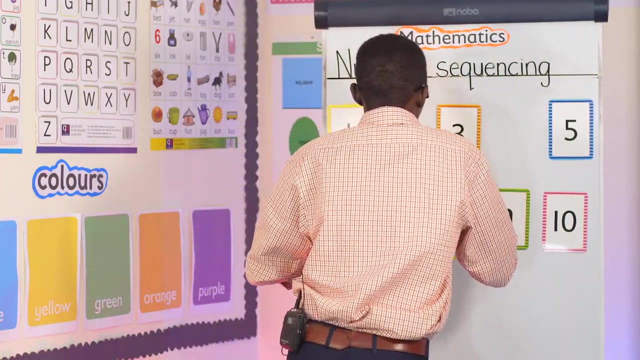 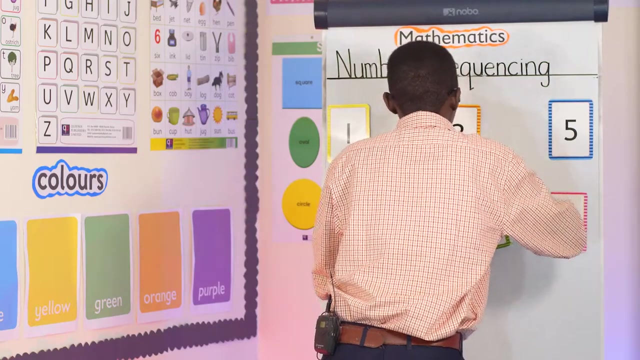 four, five, six, six, seven, eight, nine, ten. Good, Now, today I want us to do something we call filling in the missing numbers. Okay, I want to hide you like this, so that you may not see. Mm-hmm, I don't want you to see what teacher David is doing. Good, Now, look here. When you 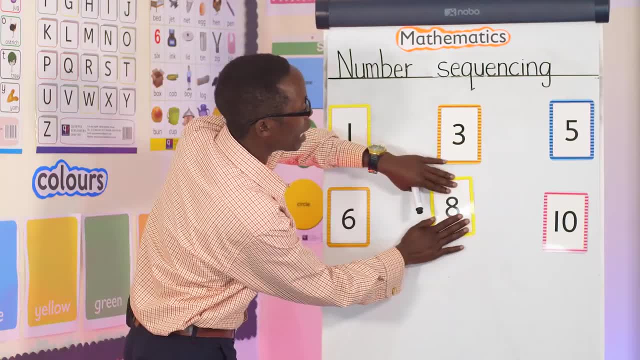 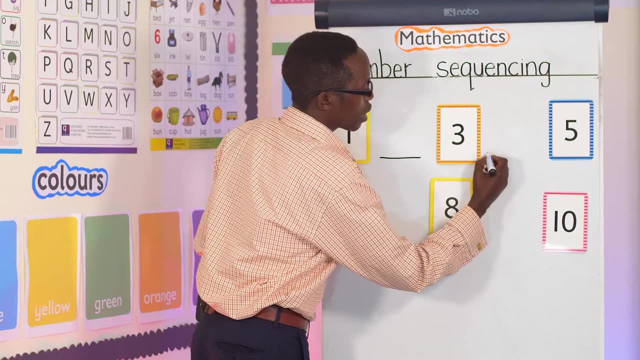 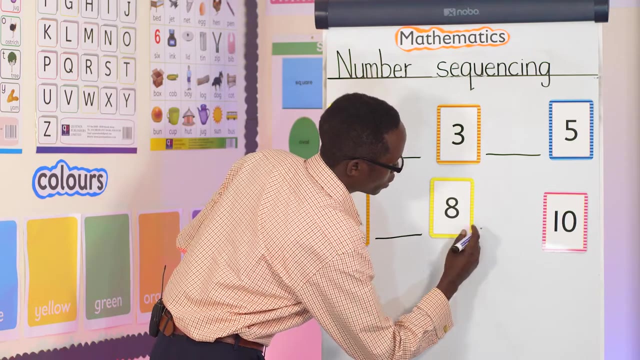 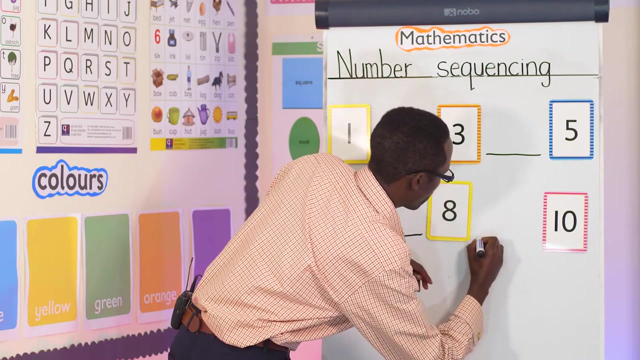 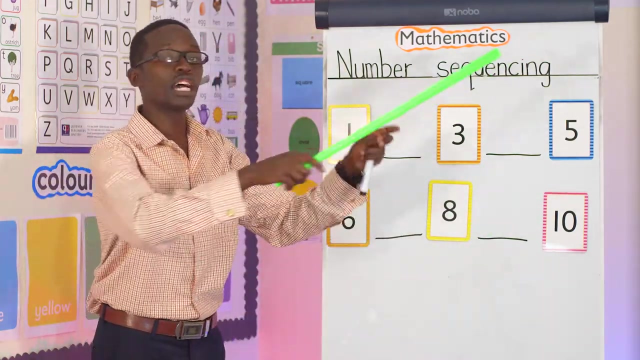 look these numbers, you find there are some numbers that they are not here. Here we have a number that is not there, Another one there. teacher have removed Another one here And another one. And another one here And another number here. Okay, Now I want us to read. Let's read these: 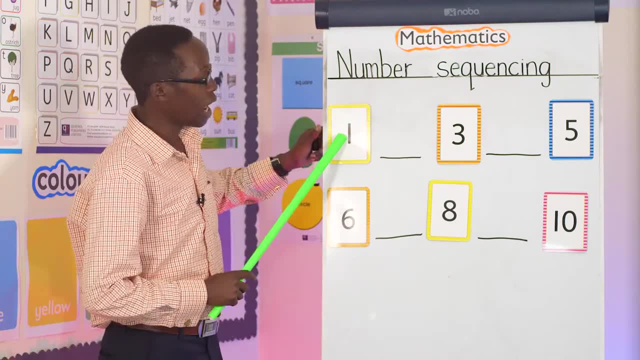 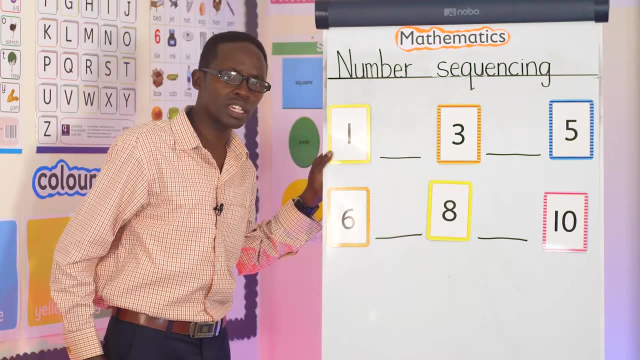 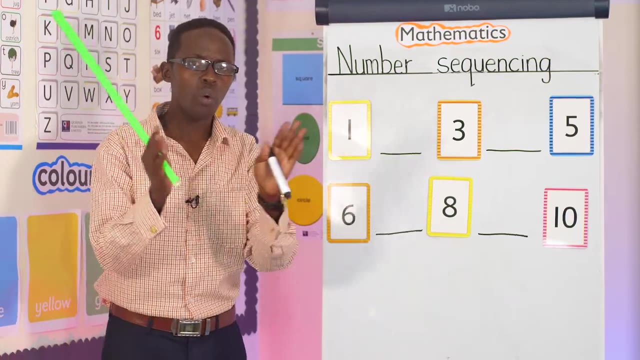 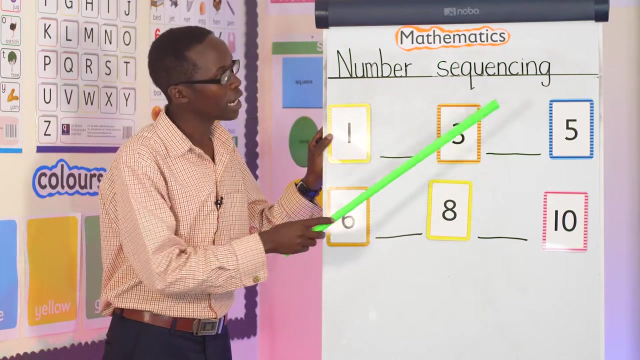 numbers on my board. Okay, One, three, five. Do we read numbers like that? One, three. Do we write numbers like that or count like that? Uh-huh, Now we say to start: One, two, three. But on my board you can see there are some numbers that. 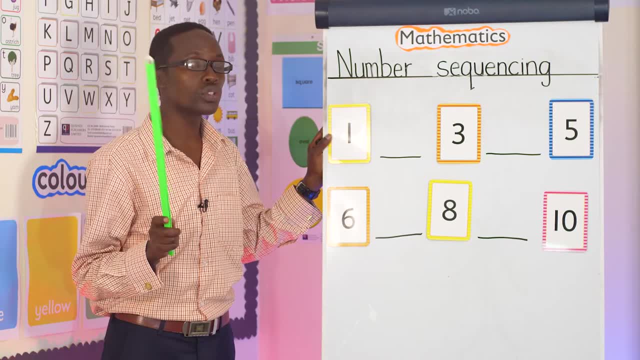 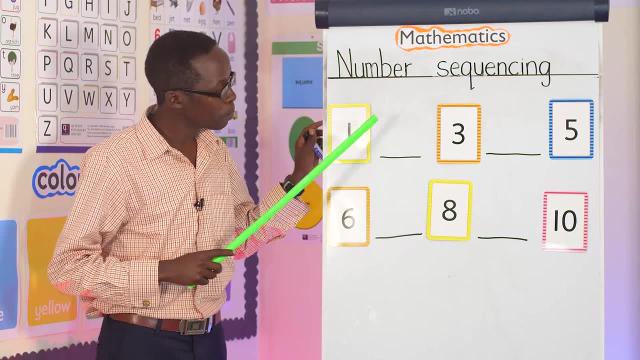 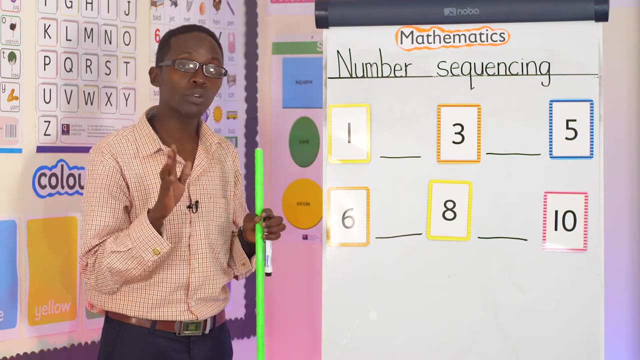 are missing. Okay, And now I want you to tell me the number. Which number is missing here? When you are told to fill in the missing numbers, you're supposed to count loudly. Okay, The way we usually clap: One, two. 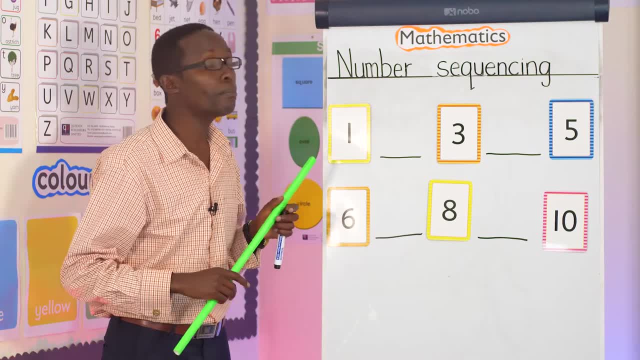 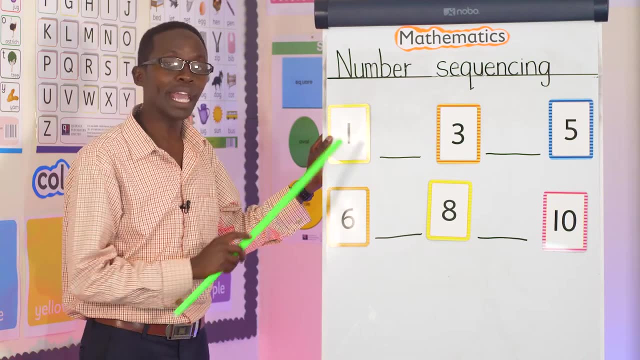 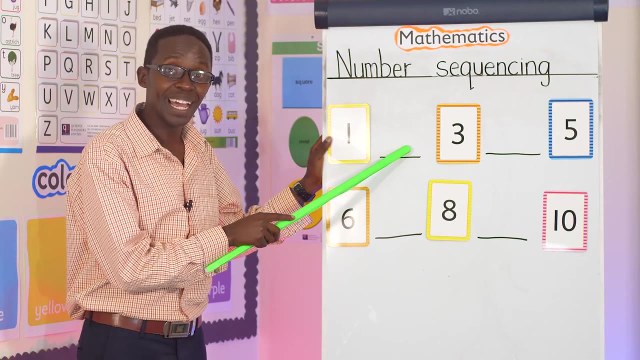 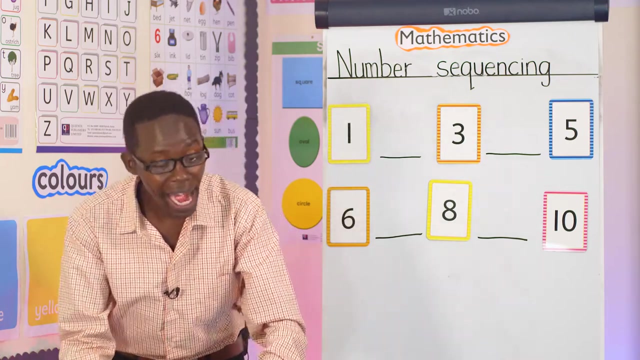 Like that, So that when you find there is a missing number, you look for that number and then you place it here. You fill in these dashes. Okay, Can you say: let's start One, two? Do we have number two here? No, So we go and look number two- Where is number two? Where is number two? Where is number two? 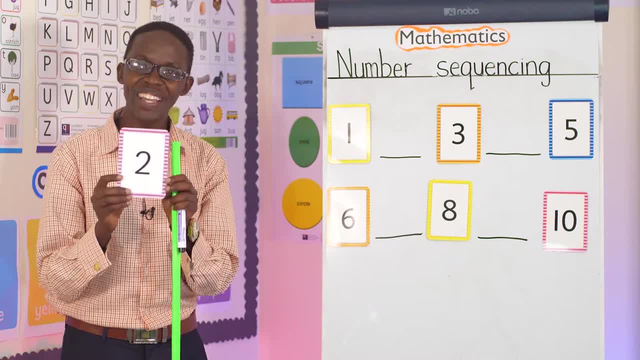 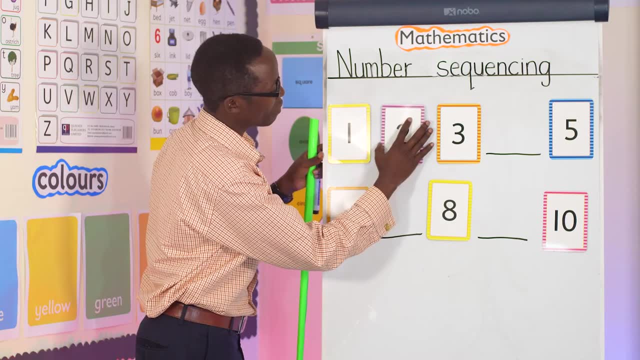 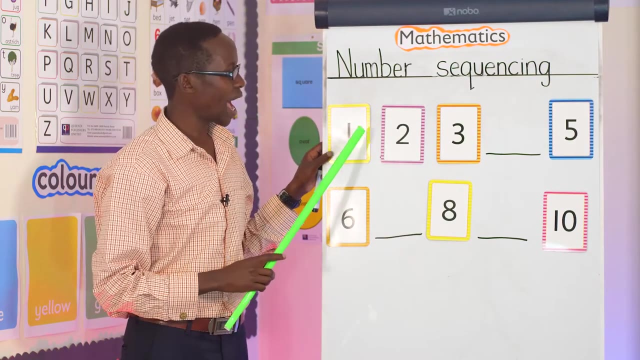 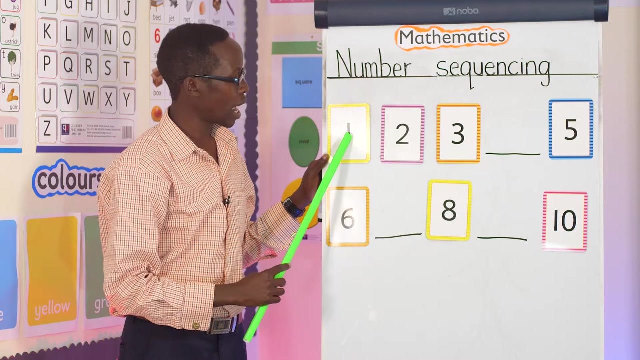 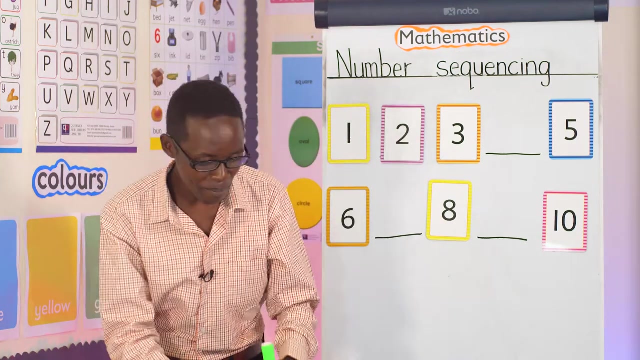 I have number two here, So I say one, two. So I come here and fix my number two. It was missing, Uh-huh, Let's start counting. One, two, three. Which number is missing here? One, two, three, Good, Number four. Where is number four? Where is my number four? 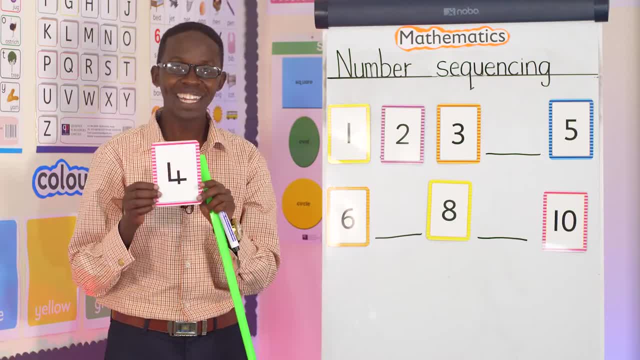 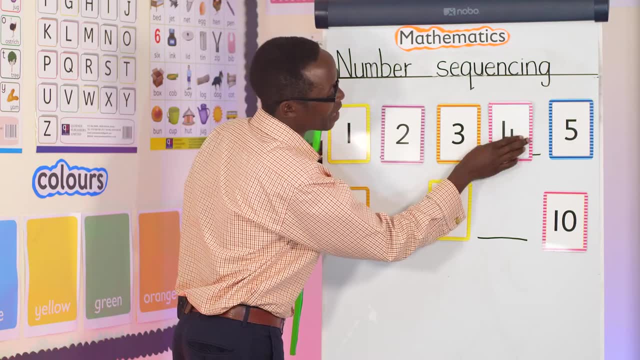 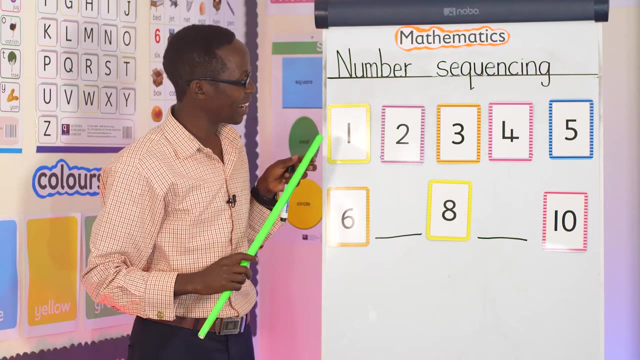 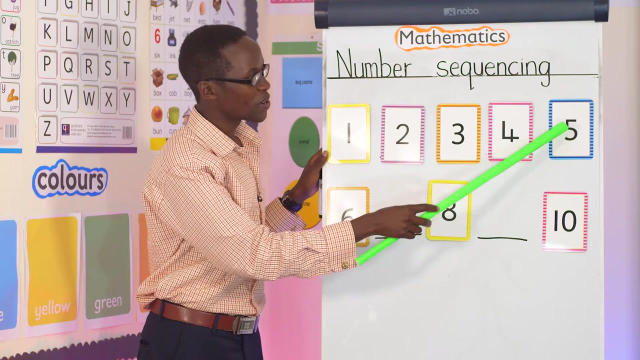 Number four, Number four. Is this number four? Good, Then you take it, You come and put there: This is my number. that is missing. My number here is missing. It is that one. Good, Let's read now. One, two, three, four, five, six. 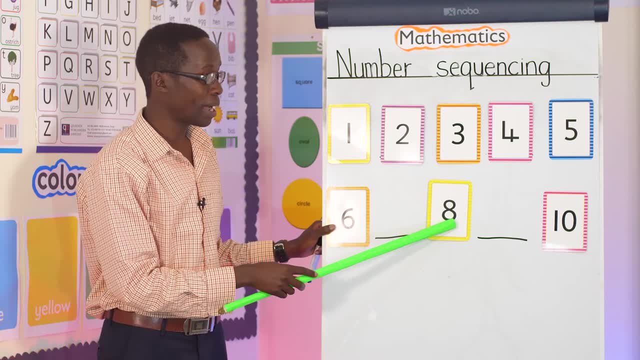 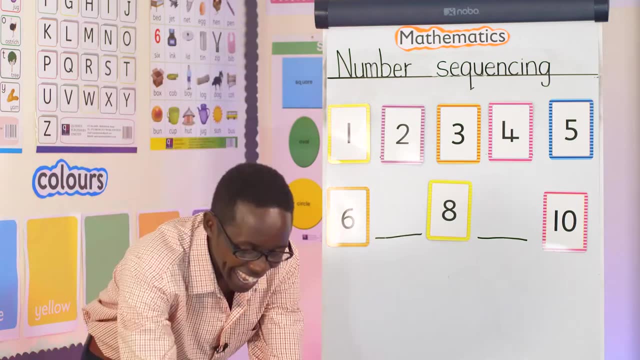 From number six we go to number. Do we go to number eight? No, Here there is a number which is missing. Six, Good Seven. I take my number seven. Where is my number seven? Where is my Wow? 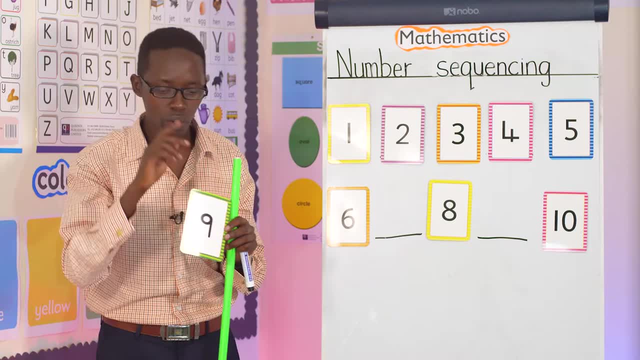 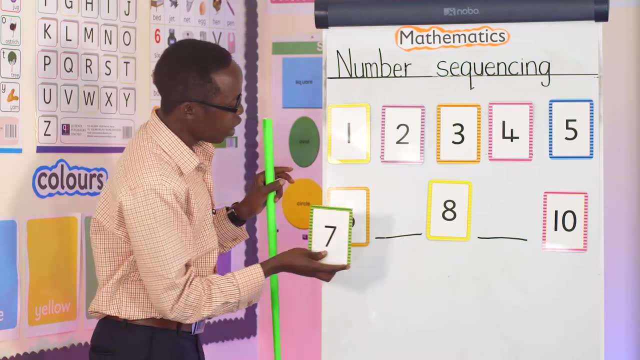 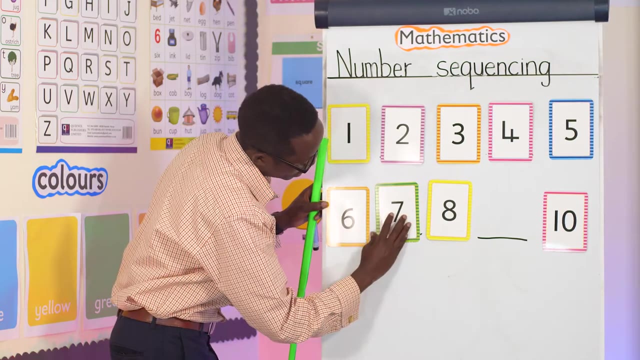 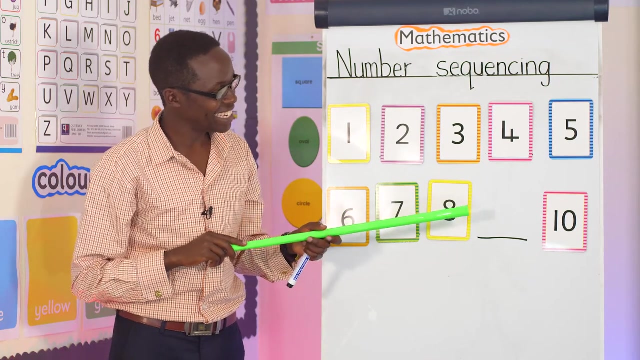 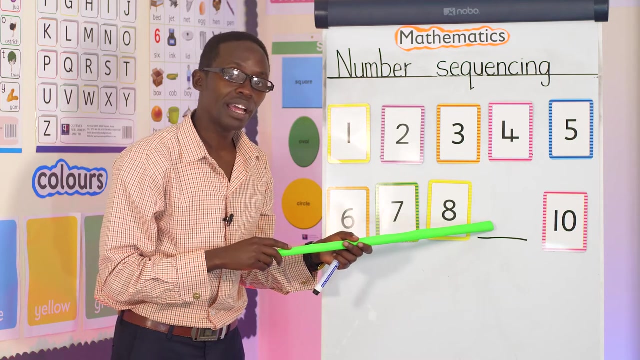 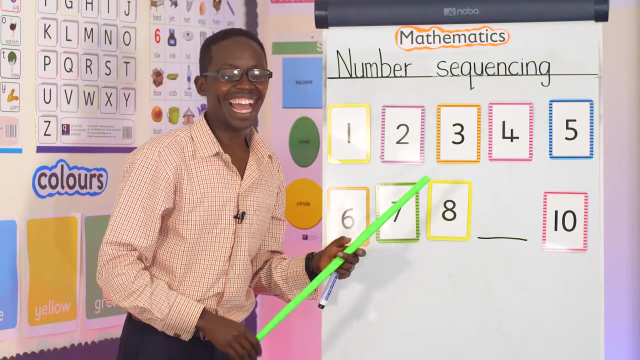 Is this number seven? No, teacher, David, That is not number seven. Is this number seven? Yes, Seven, my car Walking stick. Six, Seven. I have number seven here and you can see: Good, Six, seven, eight, I can't hear you- Eight. Then we go to from number eight, We go to number You don't know. Let's start again. Six, seven, eight, nine, Good Number nine, Uh-huh. And here I have number nine.